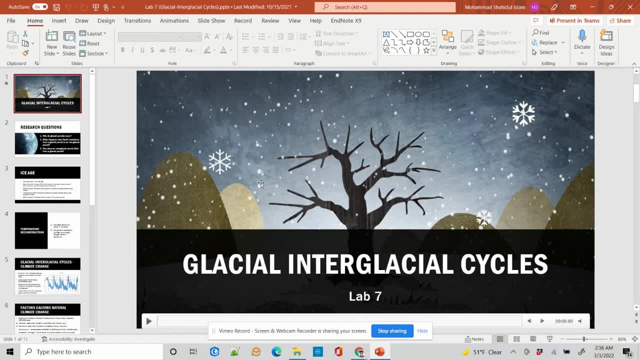 interglacial period. what is glacial and interglacial cycle and how often does they occur? how they occur, what is the time frame? and we will also see if there is any pattern in this cycle. so the research question will be based on them, as usual. so 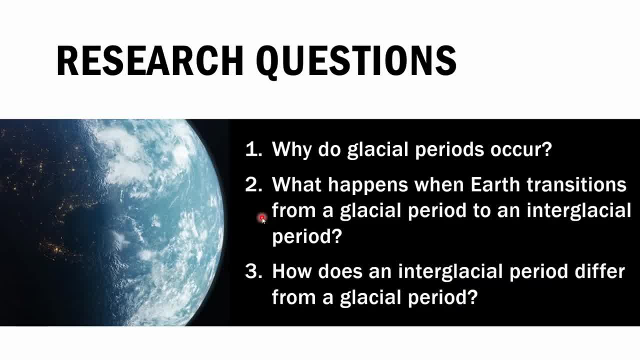 okay, let's start from the first research question. so it will actually ask about how, why glacial periods occur, how it occurs, what is the difference between glacial and interglacial period, these types of things. so, end of the lab, you will be able to answer everything related to glacial. 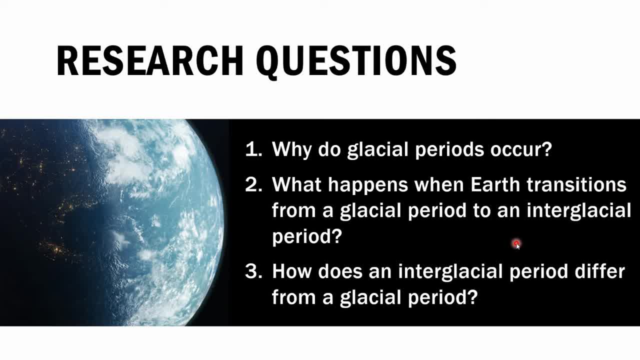 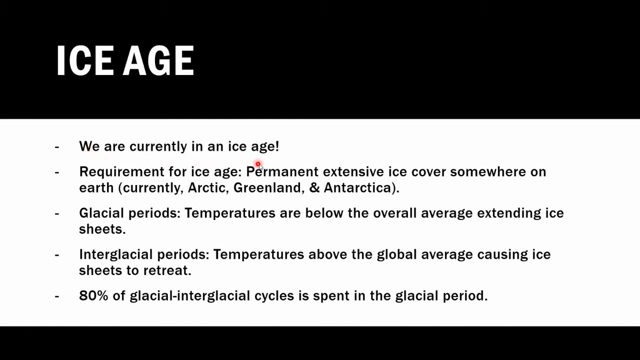 and interglacial period, and this is a comparatively demanding level. as I can, I must say this is a bit demanding lab. you will need to, at least for budget considerable amount of time for this lab, so let's go to the first slide. so right now we are currently in an ice age, even though it might seem shocking to you, but it's the. 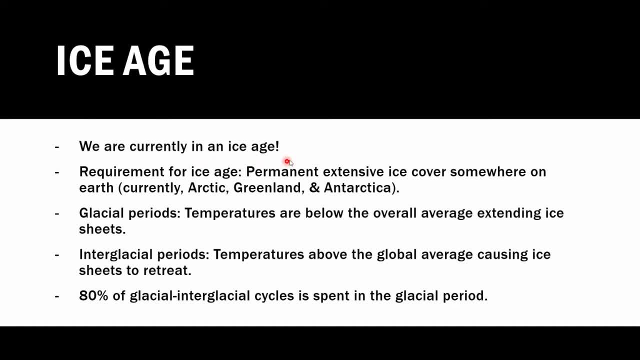 idea is that to become to be considered in an ice age, we must have a permanent ice cover, at least anywhere in the world. it doesn't have to be the whole, it doesn't have to be covering the whole Earth. at least if there is some place where we can see at least permanent ice cover, that is the prerequisite for an era to 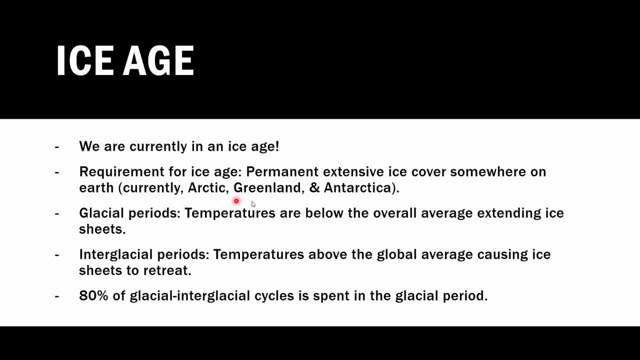 be considered as an ice age. so if you look at this in here, like Arctic Greenland and Antarctica that has some ice that doesn't melt even during the summer season, like there are some sort of ice, some thin ice that melts away during summer and come back again during winter, but there's some big chunk of ice that 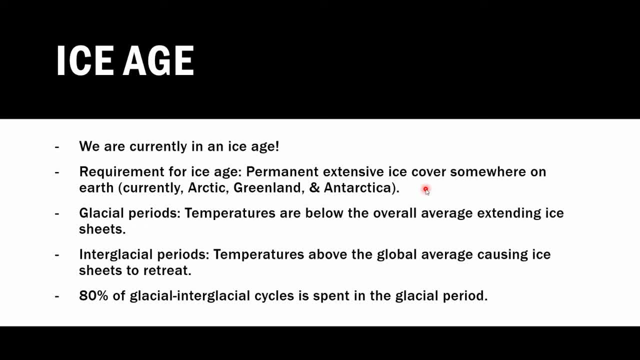 some portion of it probably melts, but it doesn't lose entirely. so that means we're still in ice age. so another point is the glacial periods. so glacial periods is a period when the temperature is below the overall average, so below the average temperature. so that means when the temperature 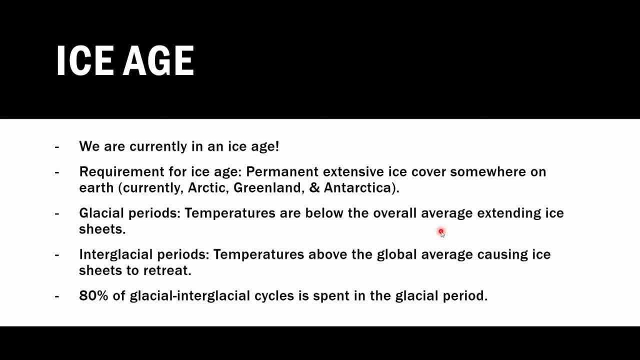 is lowest, temperature is coldest when the at surrounding is coldest. uh, that is, that is what glacial period is, and the interglacial periods is when the temperature is above the global average. so, uh, the global level. I will show you from a graph what is global average like, usually, if you 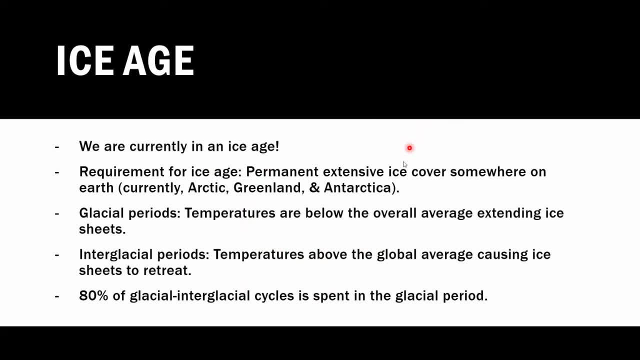 look at the glacial and interglacial cycle and the overall high peak temperature and low peak temperature, you will be able to understand. you will see that the average temperature is around minus four minus three something. so anything above minus four minus three is interglacial. anything below minus four. 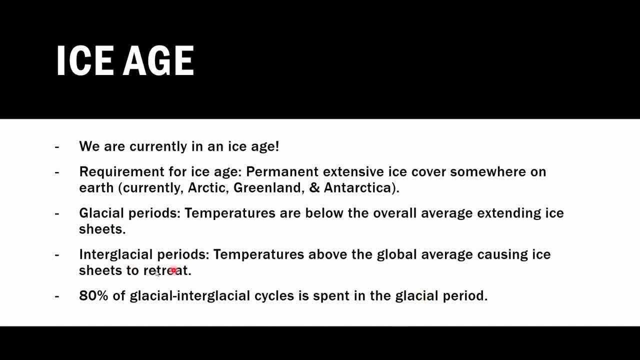 minus three is a glacial period. so, uh, one of another point is that, uh, with glacial and interglacial, um, there is that is called a cycle, which is, we can say, glacial and glacial interglacial holders. so when there is glacial cycles after that then comes interglacial cycles, then again. 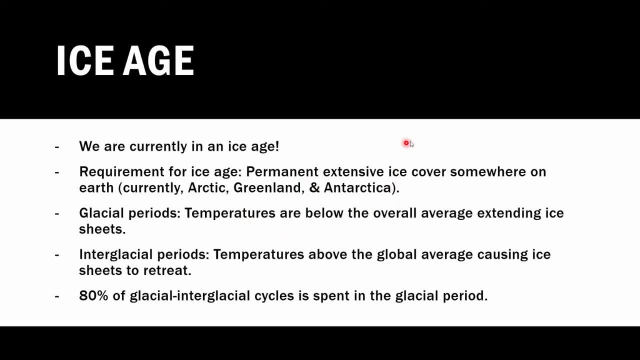 the fringe of ready shit. then come slash here, then again up to that ratio. then comes interglacial cycle. so we just take Glacial and interglacial cycle, uh and uh, consider about, consider the, about temperature and everything but among, indeed in that cycle. I will show. 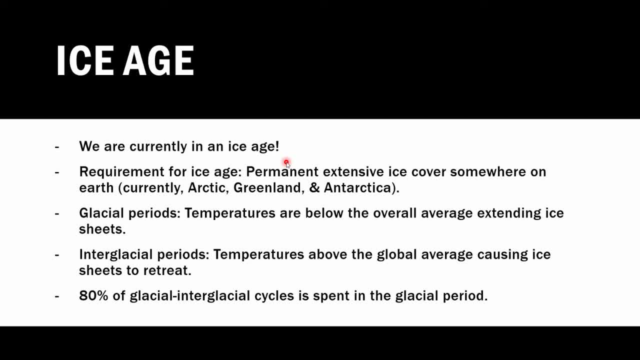 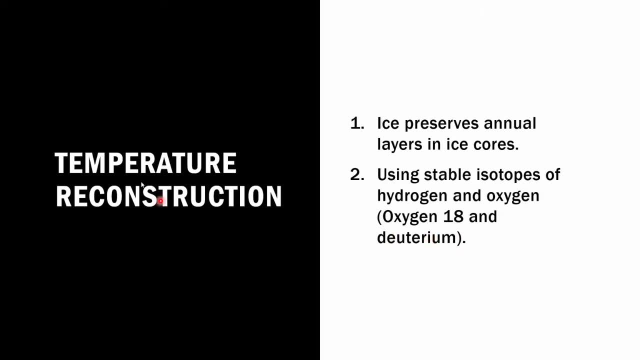 you in a moment in that cycle. most of the part is actually in the integral. so in the glacial period, almost 80%. so the next slide is talking about the temperature. reconstruction scientists figured out a way to identify the temperature from the past for around almost 450,000 years ago. how did they do? 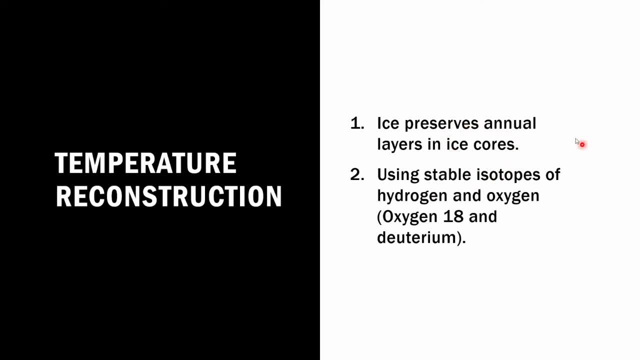 that they used ice coats. so that is your question, one which will be asking: how did scientist measure the temperature? what was the way they actually analyzed the ice core? because ice core preserves the annual layer of ice, like every year, like, if you consider from 2001 to 2022, like the tutorial is. 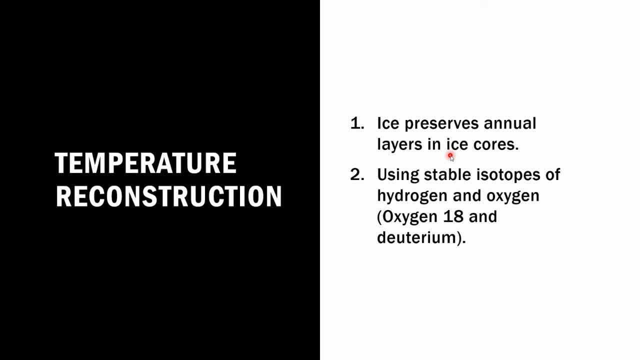 the 2001 layer is here in the bottom, then a 2001 layer will be above that 2002 level, about that 2003 layer will be about that, like it will cover one after another. so that way, when you somehow identify the 2000 years layer and you measure the composition and everything, you will. 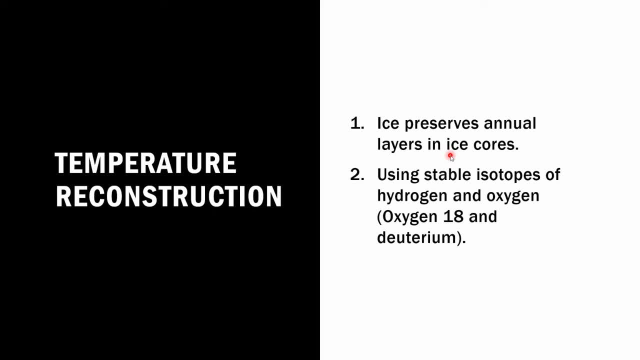 be able to understand the temperature in that layer. then you can even identify subsequent year as well and see the temperature pattern and everything. so that is how the ice core measurement works and you will be given a video to watch in the lab. so I'm not going to talk the brief about. 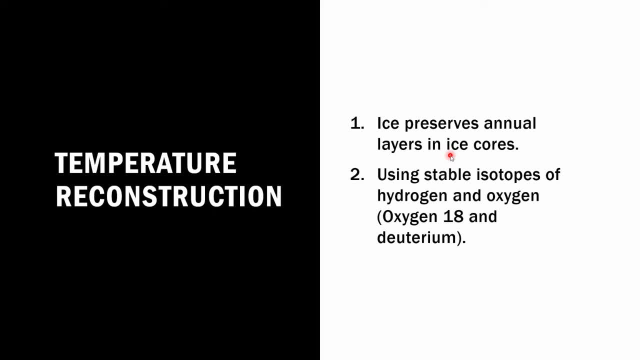 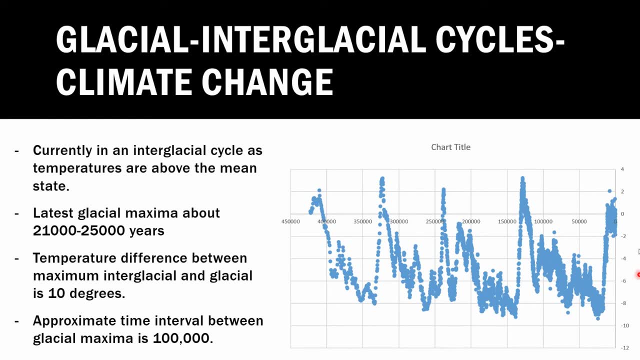 talk more about that in here, at least. next one. this is what I was talking about: the glacial interglacial cycle. so this is what: glacial interglacial cycles. as I already told you, scientists have been able to identify the temperature from previous 450,000 years ago. so right now- this is the present time there is. 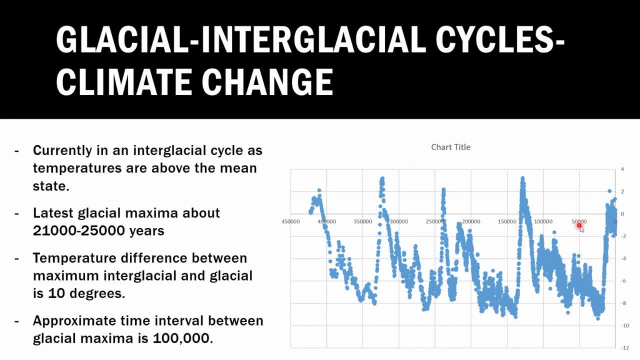 zero. that zero means now. then this is 50,000 years ago, this is 100,000 years ago, 150,000 years ago. that way they could make a temperature graph for almost 450,000 years ago. so in here Here, if you look at, if you compare the average temperature, you can see Simply Open. 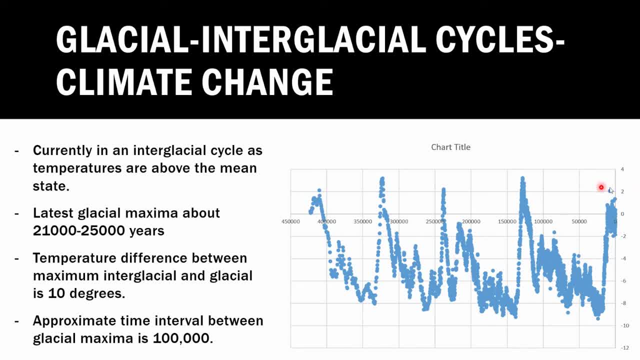 after the permeability. as you look at, if you compare the average temperature you can see from the peak, at least from this peak to the lowest peak. if you take the average of them, you'll see the average is around minus four or minus three. that is the average for us to consider. if anything is above that one, that is. 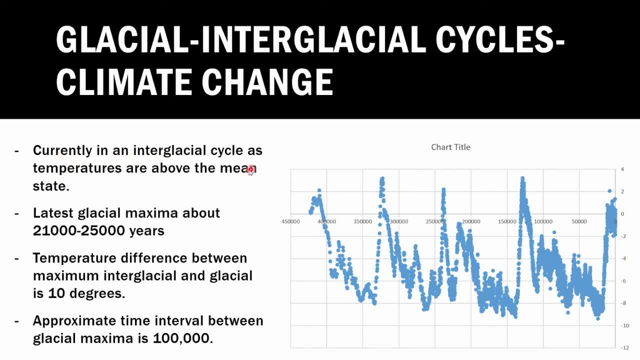 Interglacial and anything is below that one, that is clроб, so currently in an Interglacial cycle of the mean state. so right now is zero is here, which is definitely above minus four. let me use my pen tool, uh, which will help me to show you some more details. so right now we are in here. 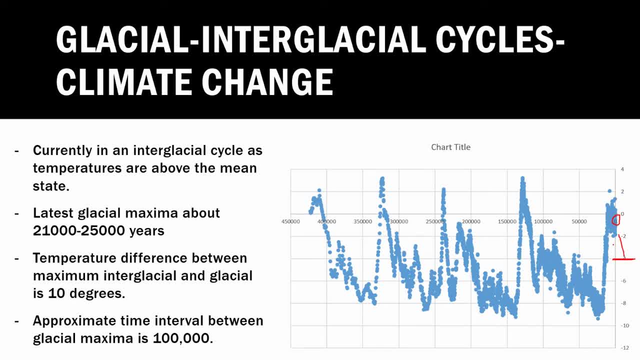 which is definitely above minus four. that means we are in interglacial cycle. if it was below, below them is the glacier cycle. so you see, latest glacial maxima is about 21 000 to 25 000 years. so before we talk about the glacial maximum, we need to know the glacial interglacial. 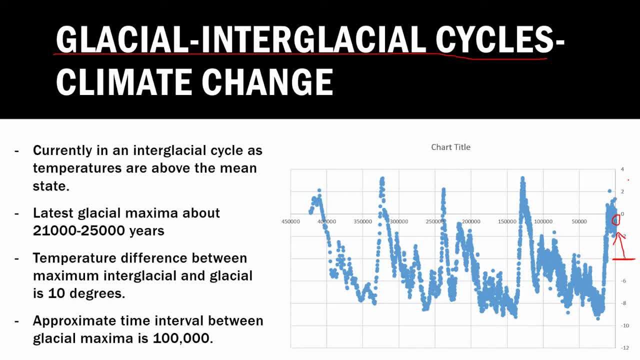 cycle. so there are around one, two, four, four and a half cycle in here, so let me show you first. so this one with the peak is the interglacial peak, the highest temperature during the interglacial period, and in here you can find the lowest temperature in the during the glacial period again, highest of interglacial, lowest of. 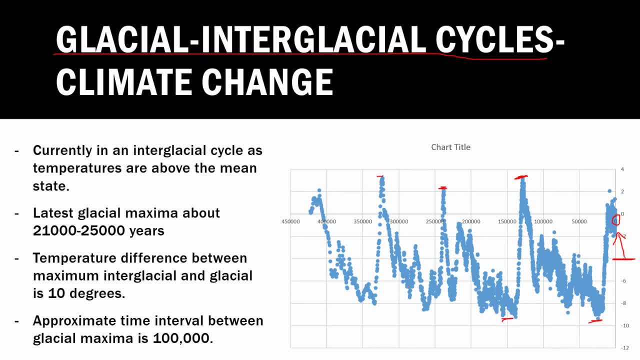 interglacial around this region: highest of interglacial, lowest of interglacial, highest of interglacial, lowest of interglacial. so that way you can find glacial interglacial cycle. you can find another glacial interglacial cycle. uh, i believe you are able to understand that now. 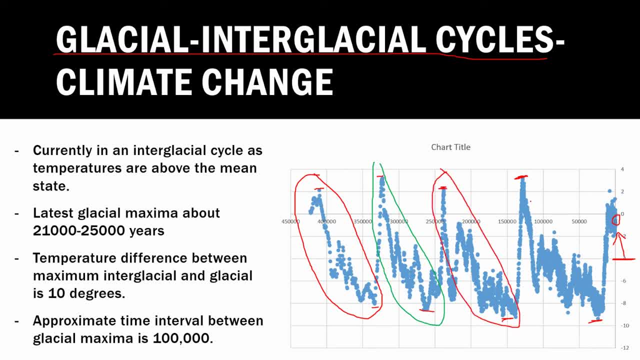 so this is another glacial interglacial cycle, this is another glacial interglacial cycle. so that way you can find, like, if you look at the pattern, you will be able to look, if you understand, get some sort of trend there, like it from here or from past, if you. 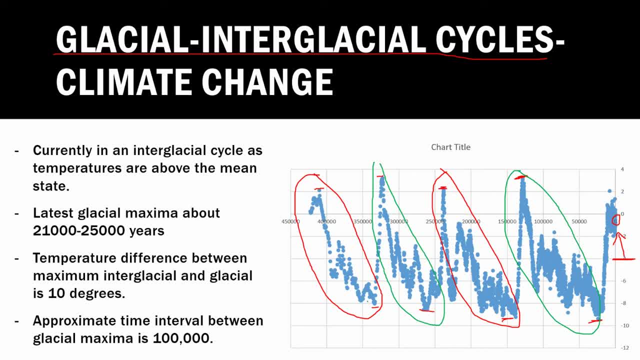 look at from the past. it went up, then it went down, down and down to the lowest. then it again started to go up and it became highest. then it went down, down, down and down to the lowest and again it became highest, lowest, highest, low. so this is how the cycle went down. so from this trend, 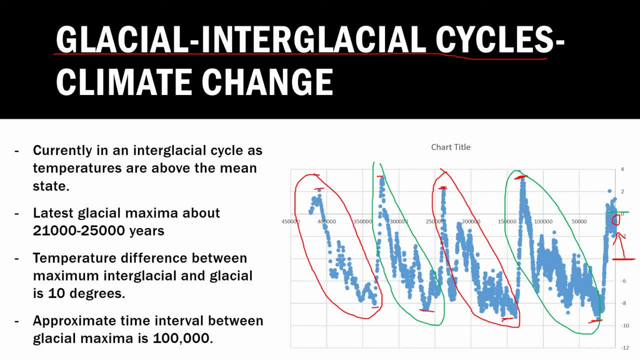 we can. we can say that we right now, we are here, so we can expect our temperature to go this to this point in the in the future, to this point around this point, and then it will go down again to the glacial cycle. so, since we are talking about this line as the mean state, 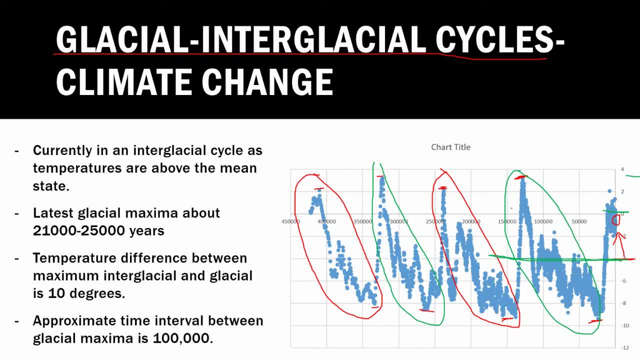 and you see, in every cycle, in the glacial, interglacial cycle, as i've already told you. so you see, the majority of the temperature is happening in this region. you see, and this region has very like steep change, but it has very small component. if you look at these as well from this line, majority of it is. 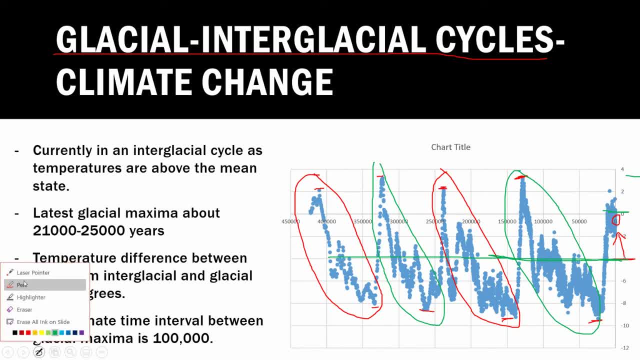 happening in the bottom, majority of it is happening in the bottom, and very few of them. so that's why we told you the previous that 80 percent of the glacial individual cycle is spanned with the glacial period. so now if we talk about the glacial maximum, so the maximum means the maximum point in 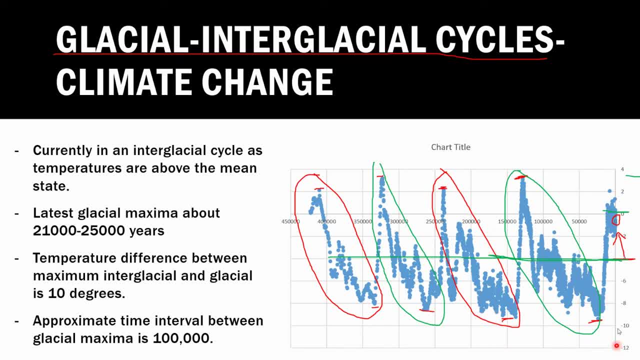 any period in any cycle. so for this cycle in here, since this region is the glacial, so the lowest one is the glacial maxima for the glacial, that is the maximum lowest it is going to be for the glacial, that is the maximum lowest it can be. so the glacial period is the lowest one, then the glacial maxima is the largest one. 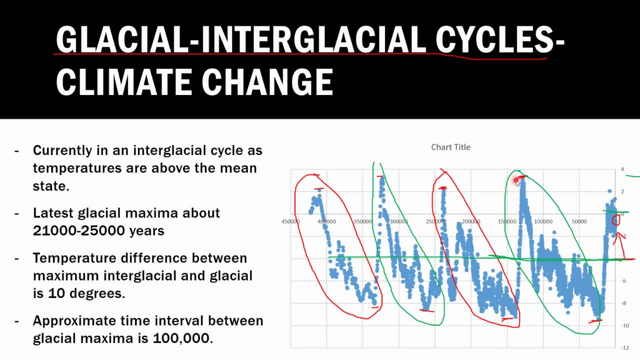 can go down. and for the interglacial, if you look at the interglacial, this is the highest maximum temperature it can go up. so this is the interglacial maxima and this is the glacial maximum. again in here. this is the maximum number of lowest temperature that the glacial period can go down. 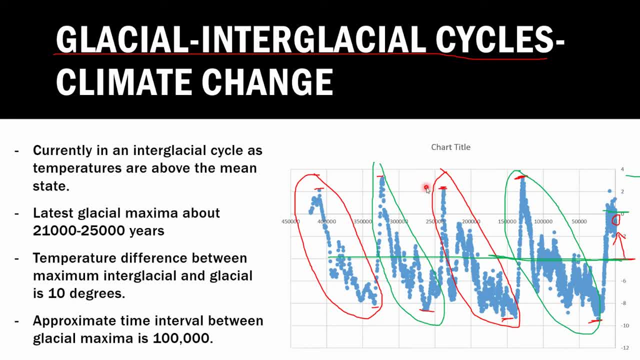 that is why it's called glacial maxima, and this is the maximum number of upper temperature that that interglacial period can go up. so that is the interglacial maximum. so when we are talking about maxima, it doesn't mean that it is maximum. it means that it is highest in its own sense, like 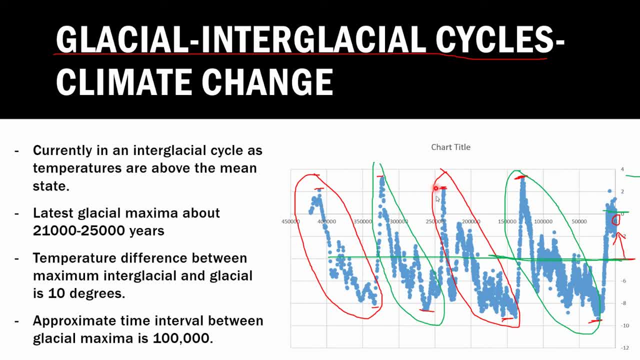 for the integration. for the highest region, it is the highest one. for the lowest part, it is the lowest one for the glacier, so that way. so if you look at the last glacial maxima, so this is the last glacial maxima that happened around. um, let me use my pen again this time. let me use 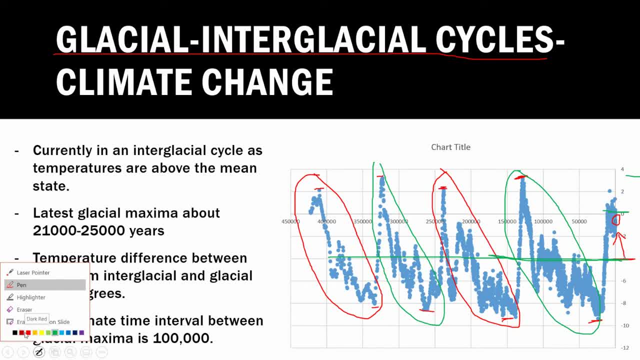 uh, what color should i use? orange red. i already used red black. let's use black black. so if you look at this and draw a line here from there, so you see it's from zero to fifty thousand years ago, so it's almost in the meat, so which we can say that that happened almost twenty one thousand to twenty. 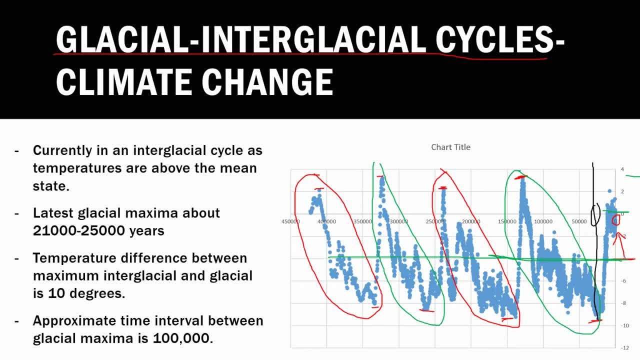 five thousand years ago and the temperature difference between maximum interglacial and glacial is ten degrees. so if you look at the temperature difference between these and that, these and that, laser again these and that, you will see the general difference is around 10 degree celsius. 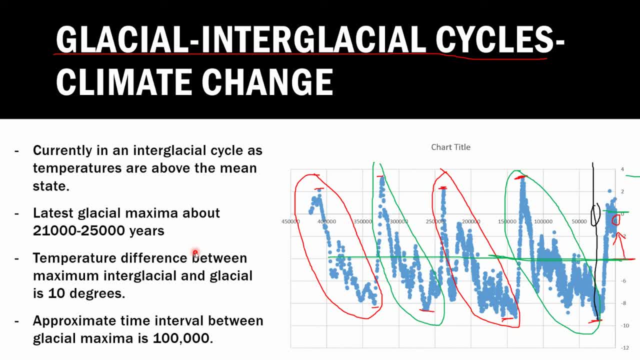 it doesn't have to be accurate. it's around 10 degree. again, if you look at the time interval between any maxima, be it glacial maxima, be it interglacial maxima, you will see the time interval is 100 000 years ago. that means if today, 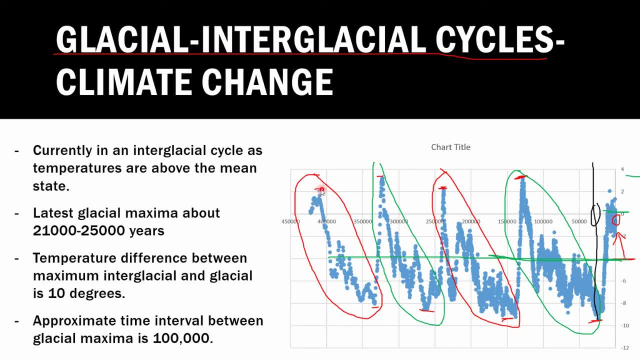 we are in the interglacial maxima. that means the next interglacial maxima will come from come after 100 000 years from today. if you look at this line in here, you see it happened around 410 000 years ago. then if you look at these: 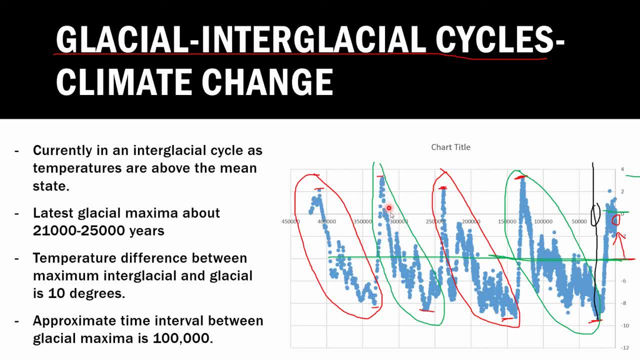 interglacial maximum. it happened around 310 000 years ago, close to that time, so that is 100 000 years in difference. same thing you can see from here, from here as well as here, so it doesn't have to be accurate, but the general idea is that the interval between each of their 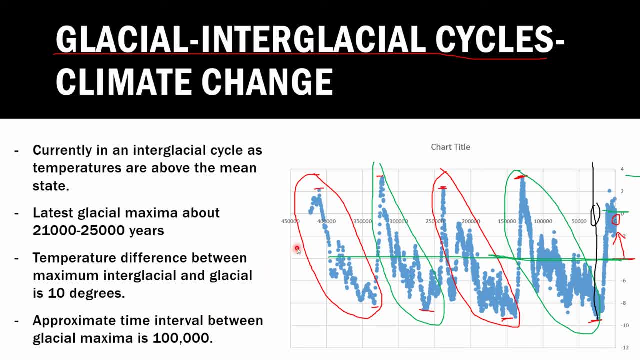 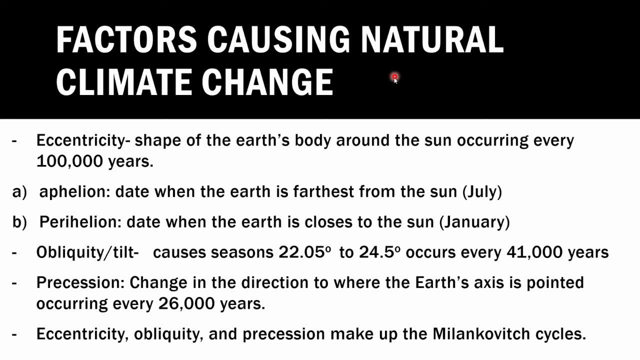 maxima is 100 000 years ago- 100 000 years. so the next slide is the climate change factors. some of those things you've studied in uh lab one, i believe uh you studied about earth tilting, so here you will also study about the arts, eccentricity. 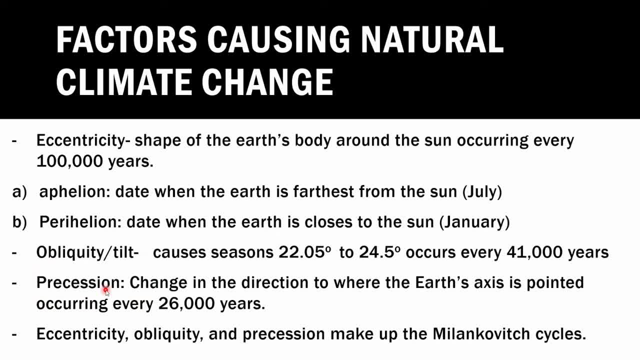 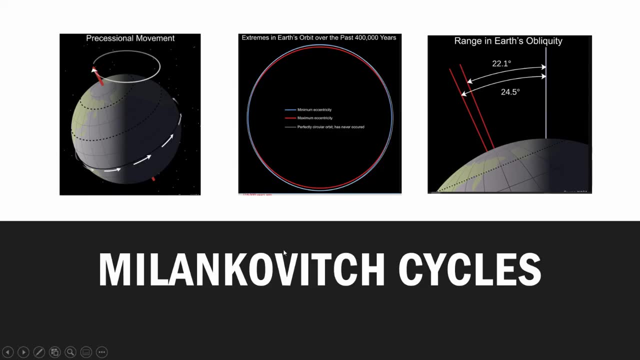 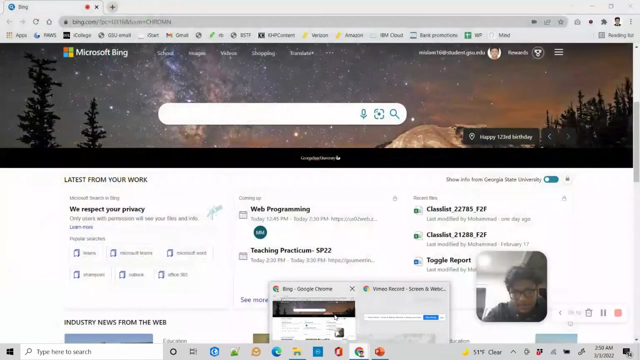 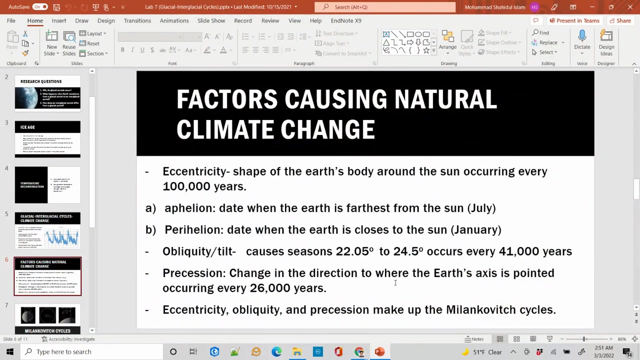 arts obligatory tilt, which you already started, and arts precision. so give me a moment. every time i work in the night, discard this. okay, let me pause it for a while. i'm just coming back. so sorry for the interruption. uh, i was hearing some sort of sound outside. this is three in the night. 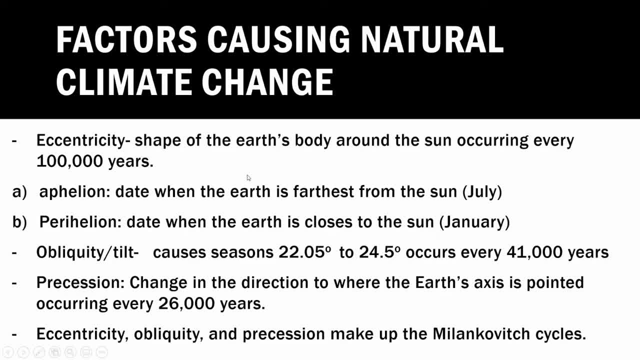 that's why any sound this time might, might seem creepy. okay, so let's get back to our work. and so the eccentricity, uh, so just follow this one, uh, i will show you those things. eccentricity, uh, obliquity, precision, in the milankovic cycle. so what is eccentricity? shape of the art's body. 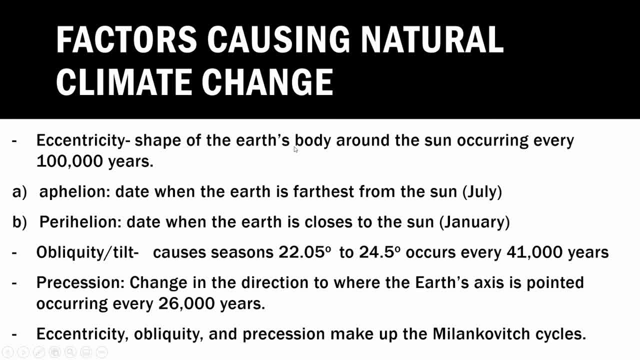 i understand occurring every 100. okay, i don't think it won't make any sense if i'm talking about the eccentricity from this, from here. just, uh, go through the term epihelion and the perihelion. i will show you a figure in the next slide about eccentricity of the keyton precision. so epihelion. 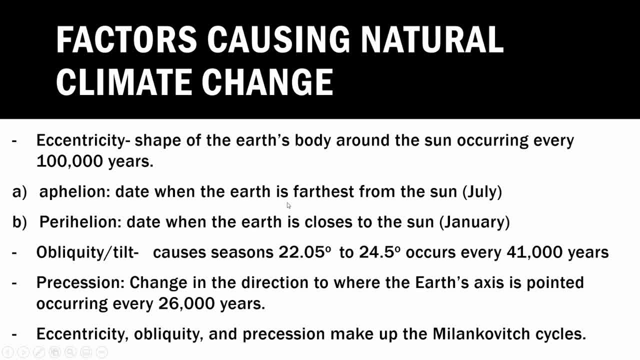 means date when the earth is furthest from the sun. that means when the sun and earth distance is highest, that is epihelion, and when the earth or sun distance is lowest, that is perihelion. so the time is there. the epihelion usually occurs during july period and occurs during january. 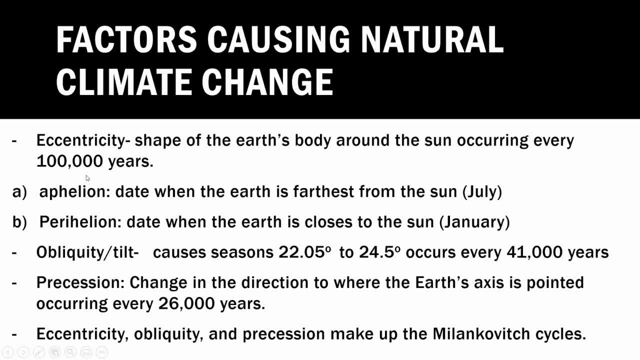 so obliquity as well as precision. so there is a eccentricity cycle is 100 000 years. uh, obliquity is cycle is 400 000 years. precision cycle is 20, 26 000 years. and eccentricity, obliquity and precision make up the milankovic cycle, which is the reason for the climate change. 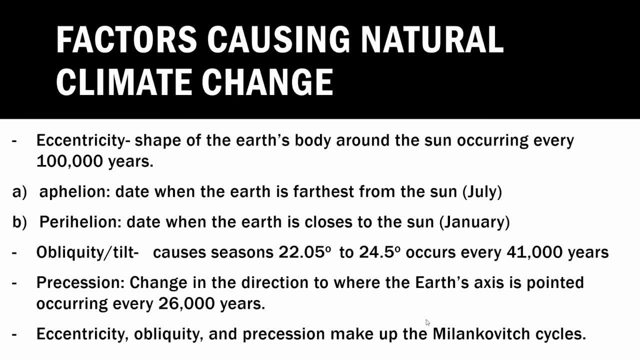 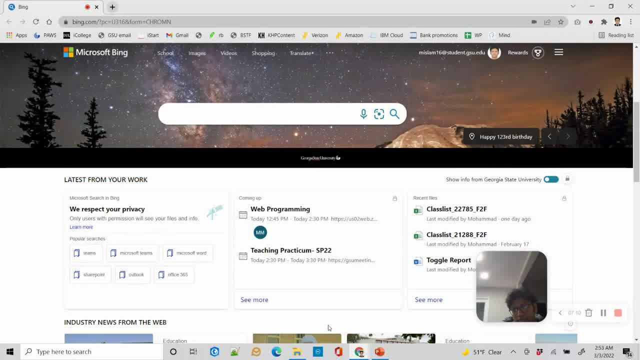 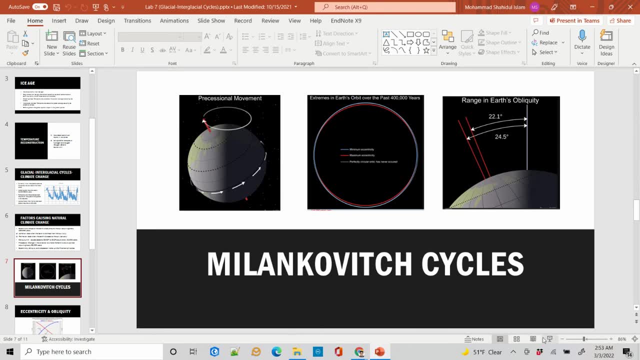 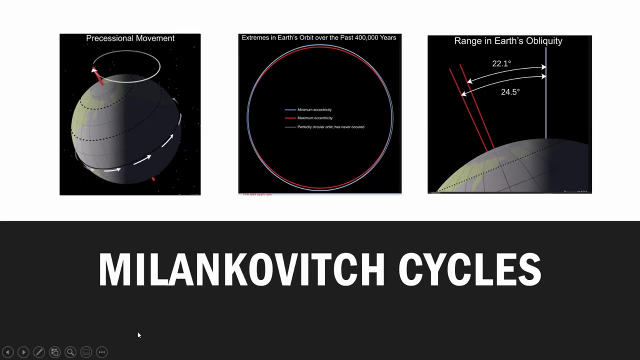 that means for these glacial periods, for this interglacial period, uh, so let's go to the next slide and see what does that mean actually? okay, so my video is running perfectly. so the next slide we're talking about. okay, so this is: uh, this is how this one works, okay. 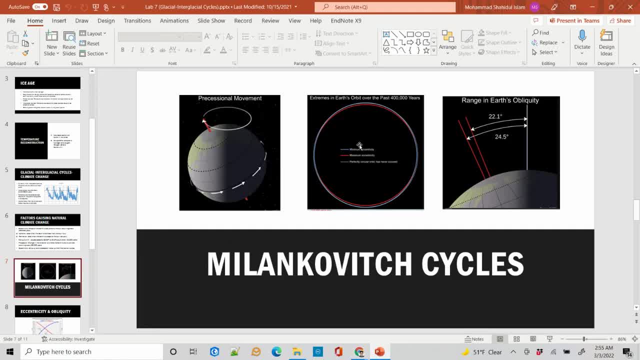 okay, so the next slide. here you can see: uh, what does it mean? uh for the precision, for the uh. eccentricity as well as for the obliquity. so uh for the precision. art rotates around this way, or use this rotation here. that is the precision, like arts axis, that. 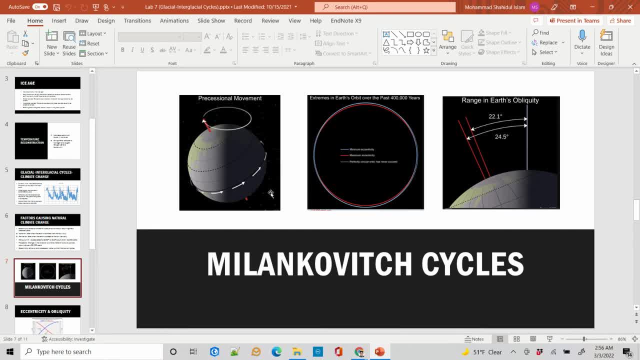 these x is actually rotors around this way. this is precision. i will show you in in the diagram, in the animation, and this is the eccentricity: some times arts orbit gets bigger. you can see the blue line. when sometimes it gets congested, you can see that in the red line. so that way, or which changes, which also 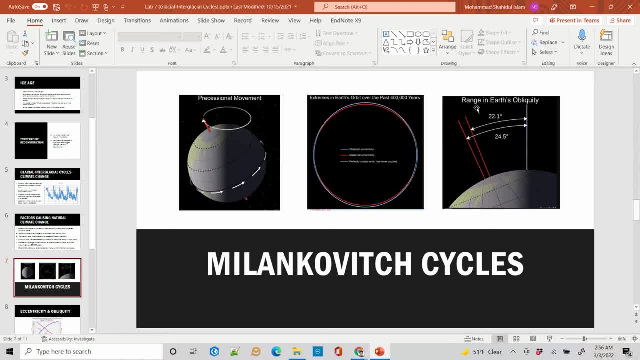 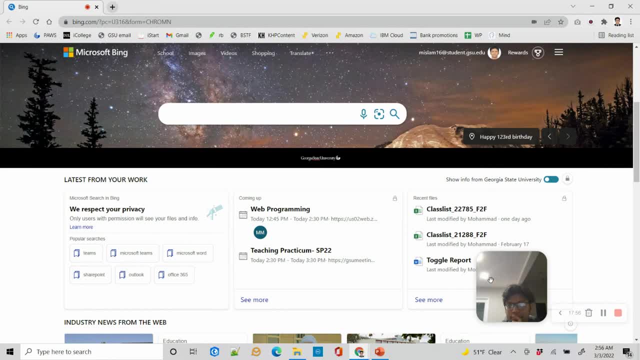 impacts some of the climate, and then, uh, the tilt. art sometimes move this way like, uh, let me show you from the here, okay. so the precision, if you- i'm not sure you can send me a hand- okay- is when art is moving like this, like, if you look at this, art is moving something. 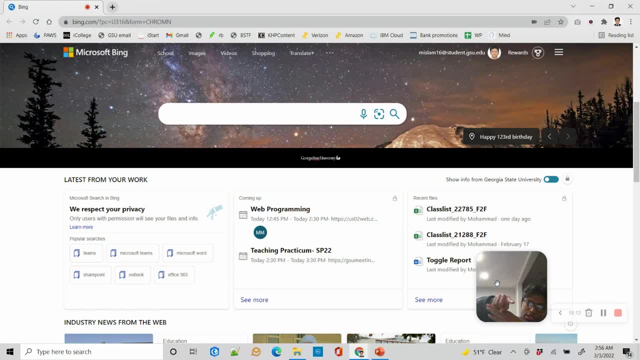 like that: this is the precision and this is the tilt, this is the tilt, like this will be the tilt. so it will look different when you look at from the side view, when you look at from the top view. so you know when I will show you the. 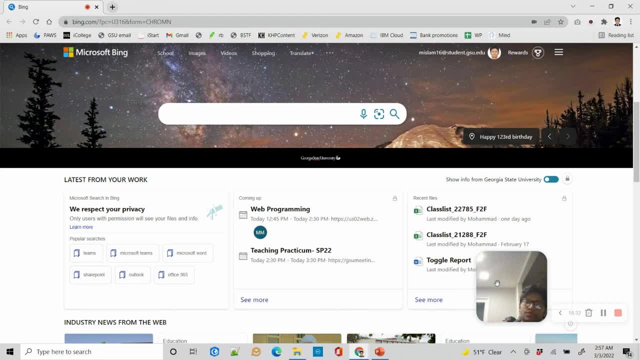 animation, you need to adjust your view according to the question to understand the movement of the art. so again, the precision arts, if that is, this is axis. this axis rotates this way, like what is in a circular motion for the tilt, it ticks like a clock, it takes like a clock up and down, up and on, something like. 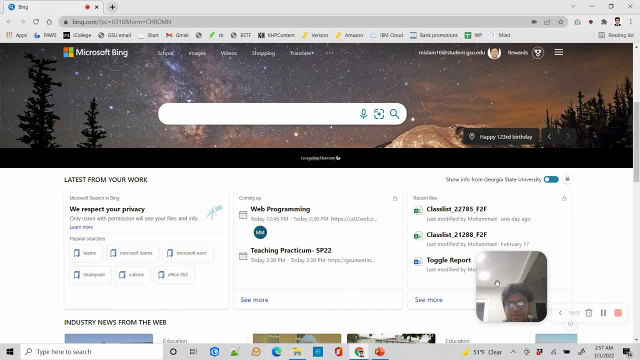 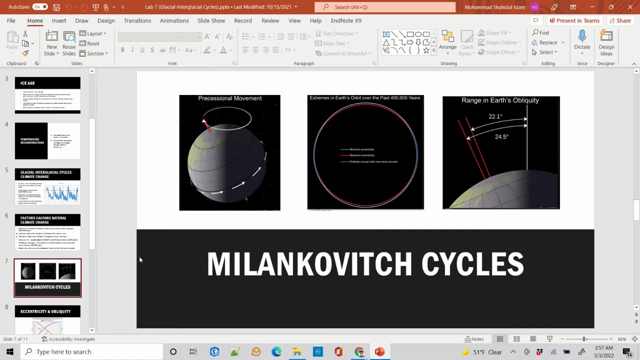 that, and the eccentricity means the orbit. if there is round, that becomes congested sometimes, that becomes expanded sometimes. so there is eccentricity. this is for I'm trying to tell it in a very simplest way, so if it might not make any sense to you, just 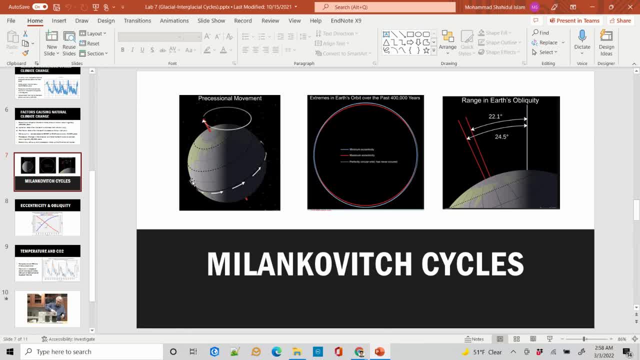 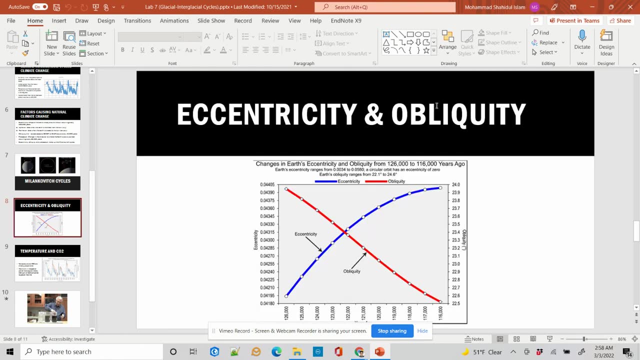 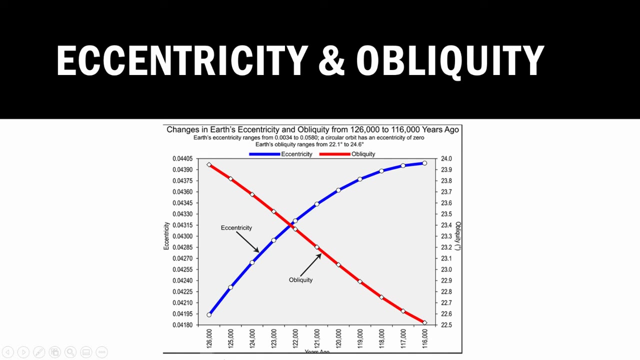 for the starter from now, we will watch that in details in our video lab videos in in a moment. make sure you don't lose all of this performance. okay, we just saw the occult on designed piece. solution of love. yeah, okay, what is it basically coloring? so This was the eccentricity. Blue line means the eccentricity. Then, 116,000 years ago, the eccentricity increased. The eccentricity increased, That means the diameter. 126,000 years ago was 0.04195 and that became 0.4405. 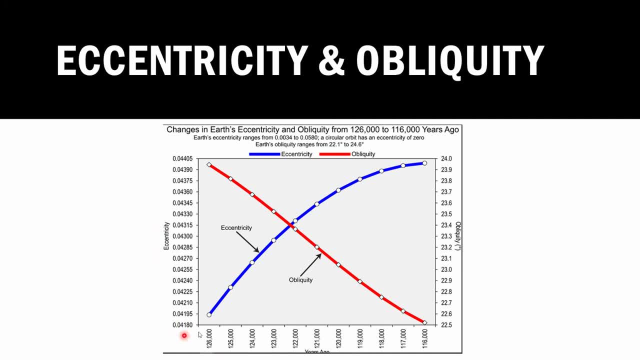 That means 0.04405,, which increased. At the same time, obliquity decreased from 126,000 years ago to the recent time, 116,000 years ago, 10,000 years later. So this is the obliquity: Obliquity at 126,000 years ago was around 24,, which became 22.5 during 116,000 years ago. 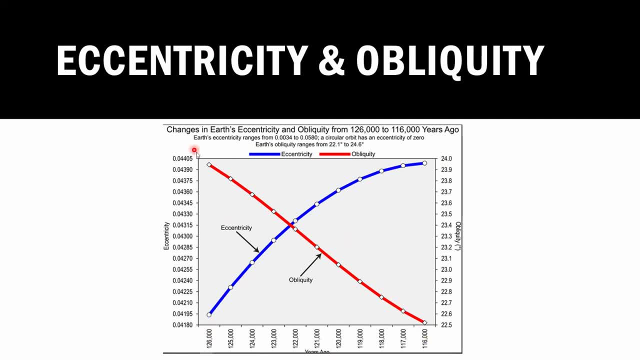 So when eccentricity increased, obliquity decreased. Obliquity means you are going to increase. So you already know that the tilting. So obliquity and tilt is the same word. As you can see from here, obliquity and tilt is the same thing. 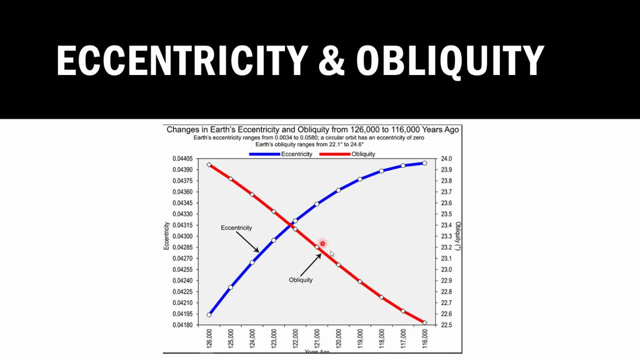 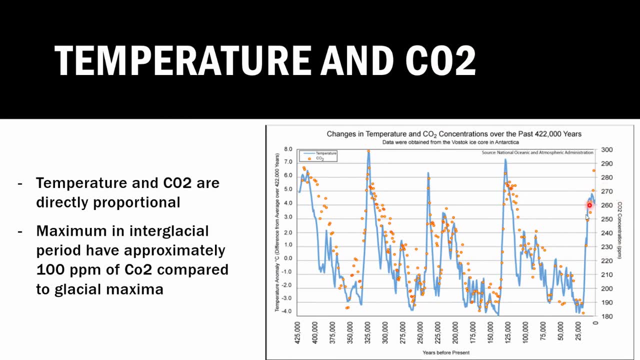 So you can just follow this graph. You will be able to probably answer two of the questions. So then there is a temperature and carbon dioxide chart. This is the temperature you already studied in the glacial interglacial cycle And now with this, 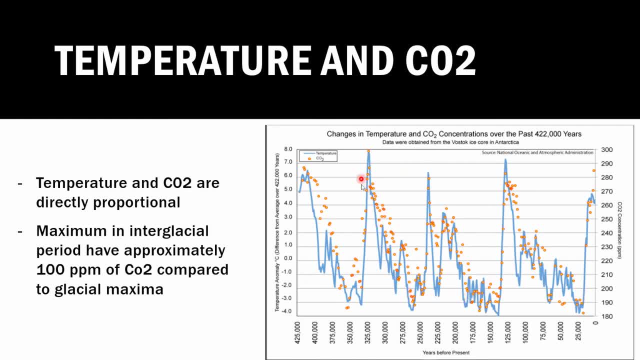 That temperature curve. they also incorporated the carbon dioxide concentration And you can see that carbon dioxide concentration is directly related to this graph. It's pretty amazing. Why is that? You see? the idea is that when the temperature is high, carbon dioxide concentration is high. 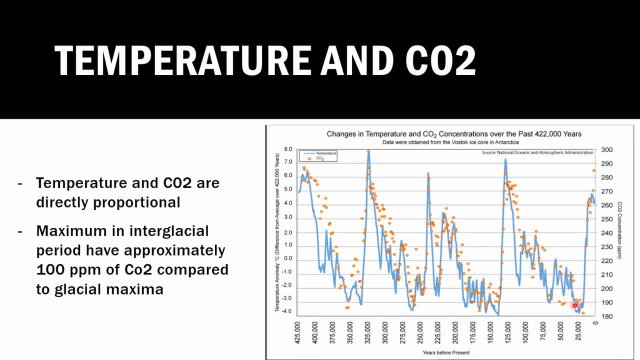 When the temperature is low, carbon dioxide concentration is low Again, in the high temperature, The carbon dioxide concentration is. you see, from this point, or at least from this point- let me use the pen tool again this point- the temperature is around eight degrees Celsius and the carbon dioxide concentration is almost 300 ppm. this is counted as ppm, 300 ppm. 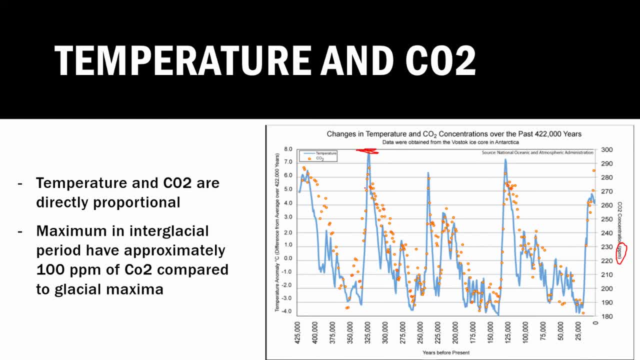 This is the maximum. Then again, when it went down, and here, When the temperature went down, Here, When the temperature is really low, minus around minus four- the carbon dioxide concentration became one eight each. Okay, so temperature and carbon dioxide due to proportion. 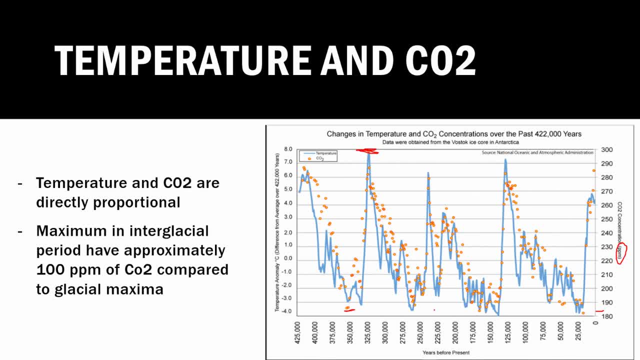 So if temperature increases, carbon dioxide increases. If temperature decreases, carbon dioxide decreases and then maximum in interglacial period have approximately 100 ppm and carbon dioxide compared to glacial maximum. So that's what I'm talking about. So interglacial period has highest carbon dioxide concentration. 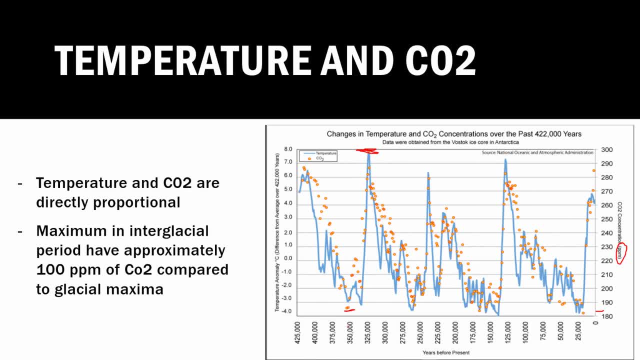 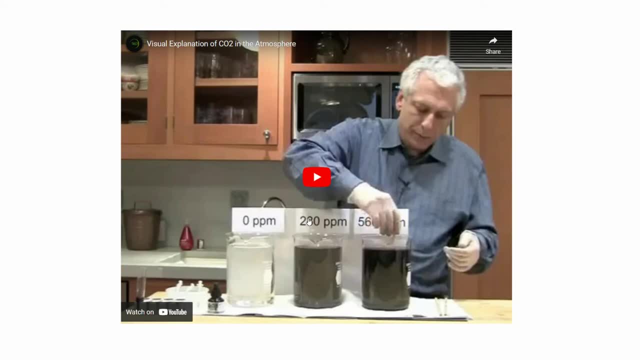 And glacial period has lowest carbon dioxide concentration and that difference can be more than or close around 100 ppm. So the next one: there is a video. just watch the video: how carbon dioxide and ppm, the calculation of ppm and how does that work.